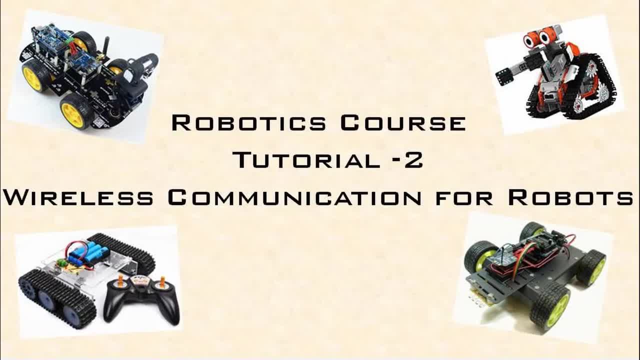 We all know Bluetooth and RF wireless methods are commonly used for making simple wireless robots. Do we have any other wireless method? If so, how efficient they are? In this tutorial 2, we are going to see what are the different wireless methods to make wireless robots. 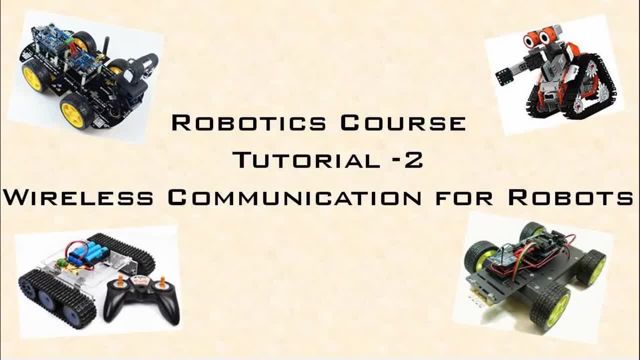 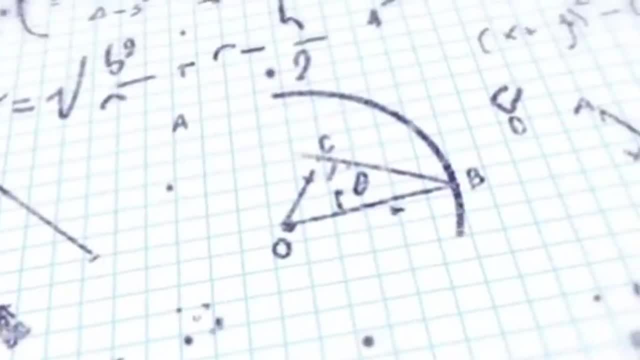 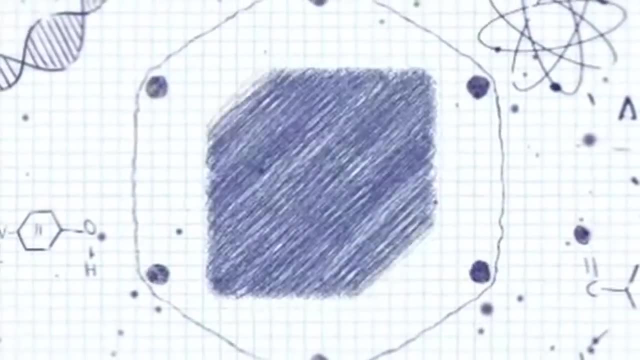 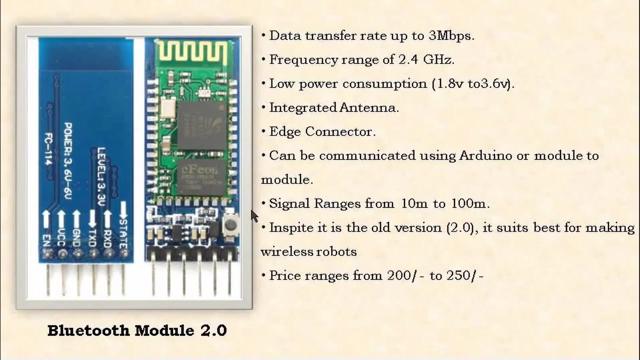 Hey guys, welcome back to Engineering Box. I am Teyesh. Let's get started Coming to the first module in wireless communication. If you search for any how to make a wireless robot, The first thing you will see is a Bluetooth, because it is very easy to make and coming. 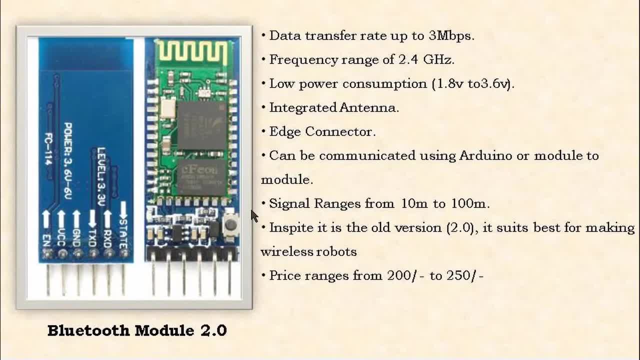 to the technical specifications of Bluetooth module. It has data transfer rate up to 3 Mbps. That means it will transfer serial data or digital data up to the maximum rate of 3 Mbps. And next is a frequency range. It has frequency of 2.4 GHz and low power consumption from. 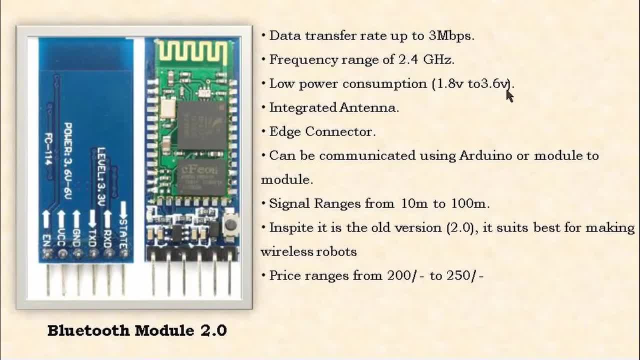 1.8V to 3.6V. Bluetooth module can be operated in between these voltage range. And next is integrated antenna. If you observe this image, you have an antenna over on the board itself, So that is called integrated antenna. 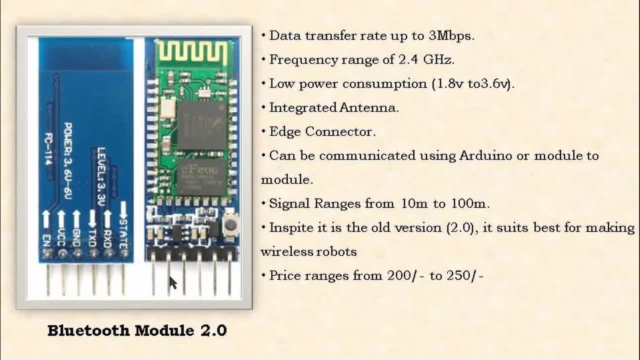 And the next is edge connector, which is used to connect to the Arduino, Can be communicated using Arduino or module to module. That means either you can use one module And use Android applications to control the Bluetooth module, or you can convert by using two modules. 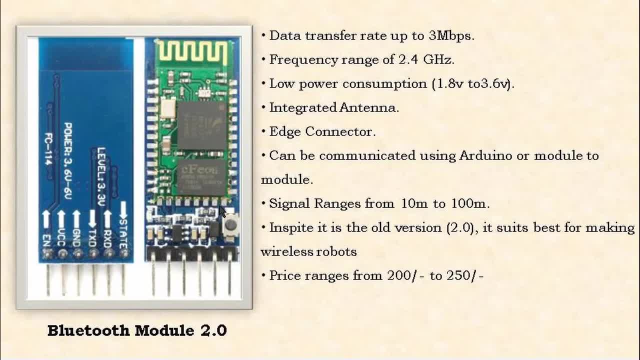 You can convert one module to master mode and another to the slave mode and give the digital inputs to the master module and that master module transmits the data to the slave module And that's how the communication is done. And coming to the signal ranges, it ranges from ten meters to 100 meters and in spite it is the old. 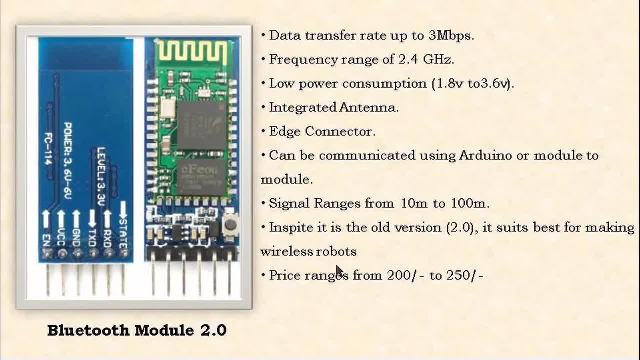 version it suits best for making wireless robots, Even though many advanced versions of Bluetooth modules are available. this is best suitable for making wireless robots because it is very easy And, last but not the least, price ranges from 200 to 250 rupees. So this is the best price range for making wireless robots And, the last but not the least, price ranges from 200 to 250 rupees. 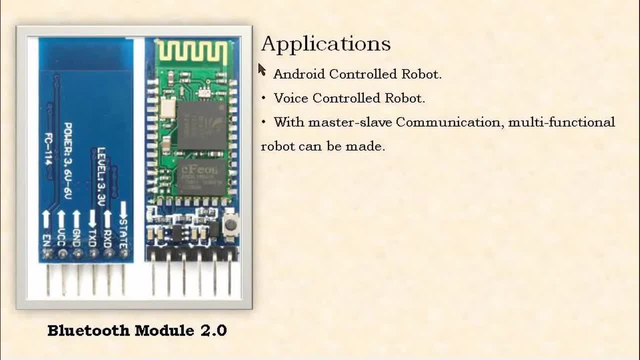 is, of course. the next is applications of bluetooth module, android control robot, voice control robot. with master- slave communication, multi-functional robot can be made. that means, as i discussed, converting the bluetooth module into 80 command mode: master, master module and slave module. we can increase the number of channels and can make multi-functional robots. however, we'll be seeing. 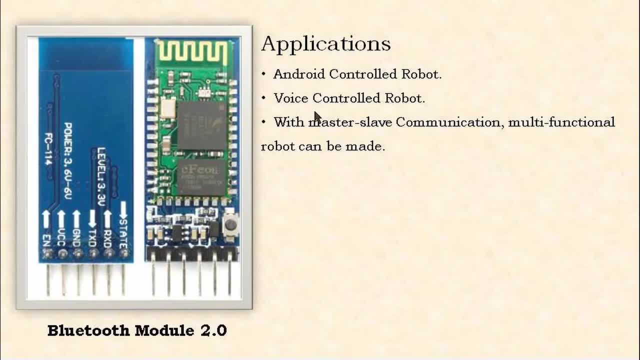 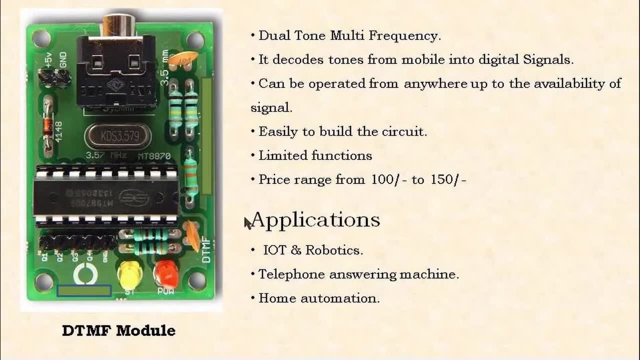 all these diy android control robot and voice control robot you'll see in the future, future videos. coming to the next module, wireless module, dtmf module, which is called as dual tone, multi frequency uh dtmf is generally used in the daily life, also if you call a customer case. 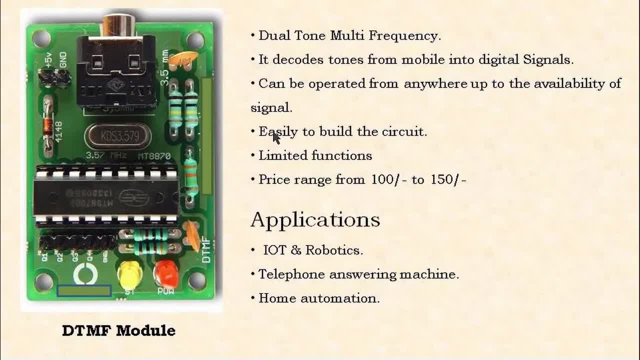 here. you won't be allowed to directly talk to the customer executive. you will be asked to the. you'll be asked some options and asked to press some numbers. that is because each number on your keypad generates a particular tone. there in the dtmf systems, those tones are converted into digital. 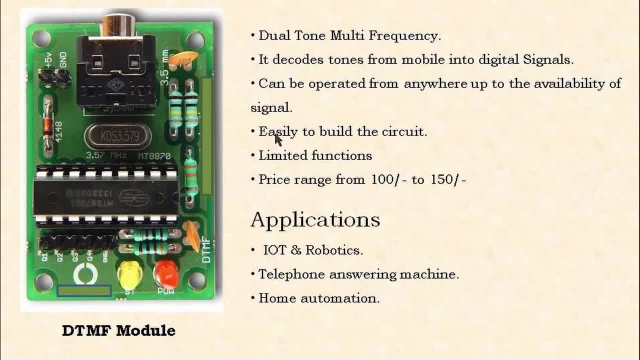 signals and that principle is used in making dtmf robots also, where this module will be converting or decoding the tones into digital signals and will be giving the output. if you observe this model, d1, d2, d3, d4 are the output of the module with the tones given to this audio jack. 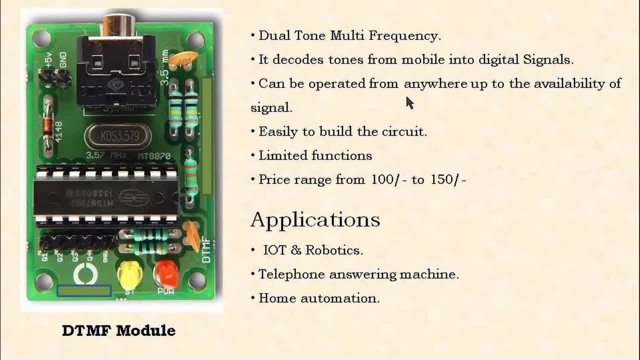 and this can be operated from anywhere up to the availability of signal. that means these are operated using mobiles within the signal range. you can operate this dtmf module. that means if you make a dtmf system and place that, place that in your home and you can call that dtmf system as a mobile is connected to that dtmf system. 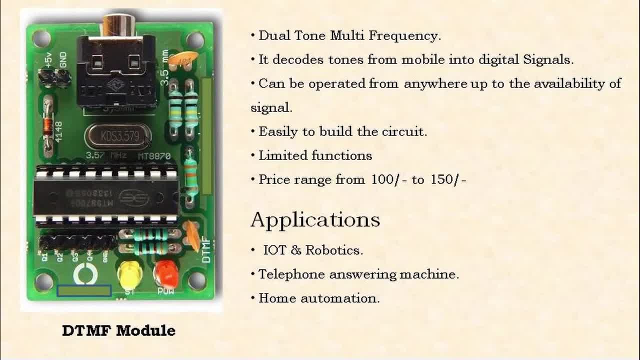 you can make a call from anywhere and control that system, the given program or anything that you have set, and it is easy to build the circuit. you can also prepare this circuit and i'll be showing you in the coming videos, and it is limited functions because it is actually operated using numbers. 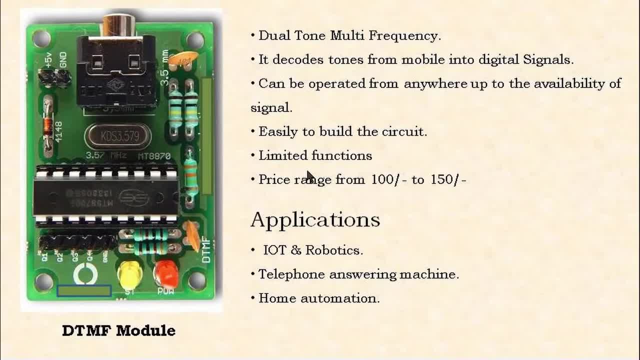 few numbers will have same tones and that will give the same digital output. so it has limited functions. if you- uh, if you are pro in writing program, you can make a, you can increase the number of functions. and the next is a price range. it ranges from 100 to 150 rupees and coming to the 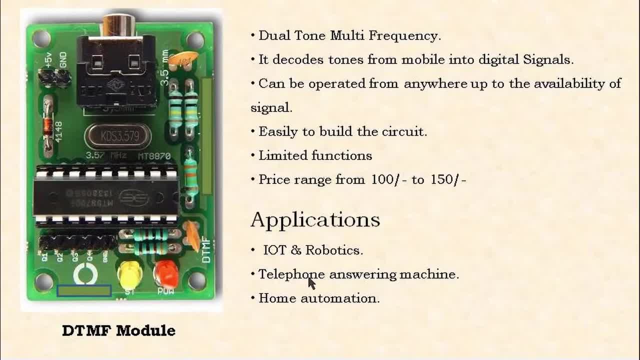 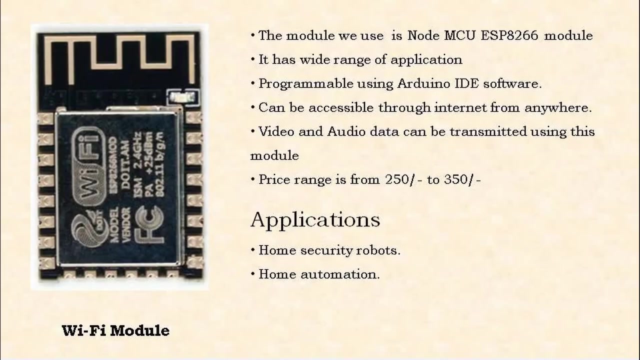 applications you can use for iot and robotics, telephone answering machines, as i explained before about customer calling, and next is a home automation or home security also you can make and that's up to you. and that's about dtmf module. now we'll go to the next module. next is a wi-fi module, as you see here, the module i. 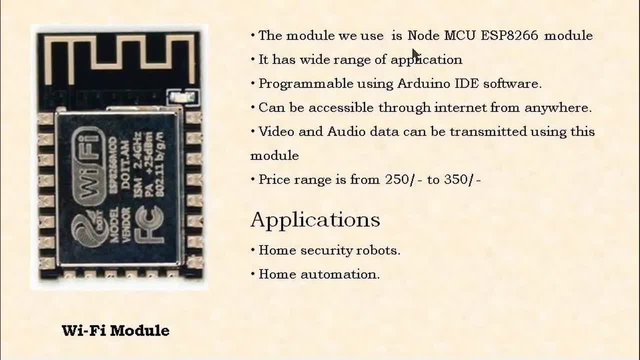 have show. i'm showing you is a node mco esp8266 model, which is a famous module and it has a wide range of application. of course, it is a wi-fi module, right? you can connect this module to your internet and you can also connect the module to the wi-fi and can transmit data, or you can upload. 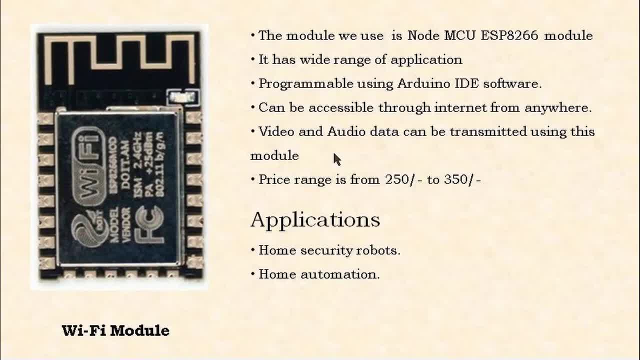 the data to the internet and you can check that data over internet from anywhere, and it is programmable using arduino ide and this can. this is connected to the arduino and you can program the module. this can be accessible through internet from anywhere, as is a white five wi-fi module, the 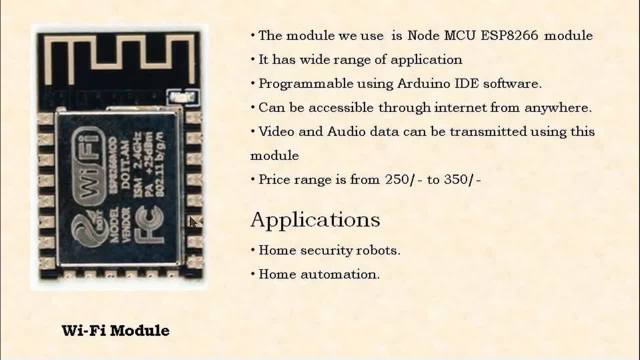 data is uploaded, uploaded to the internet and next, video and audio data can be transmitted using this module. yes, and if you, if we connect audio or audio microphone or any spy camera or gopro camera, the data is uploaded onto the internet. the price range of this module is from 250 rupees to 350 rupees and coming to the 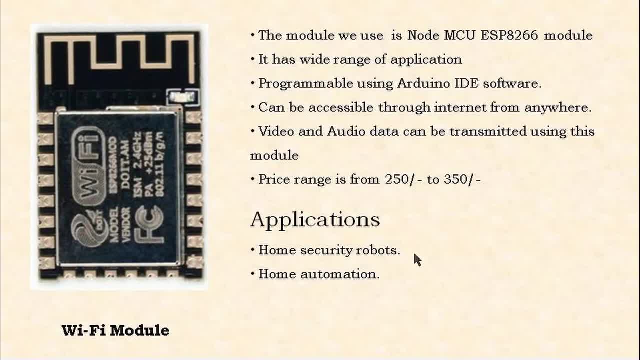 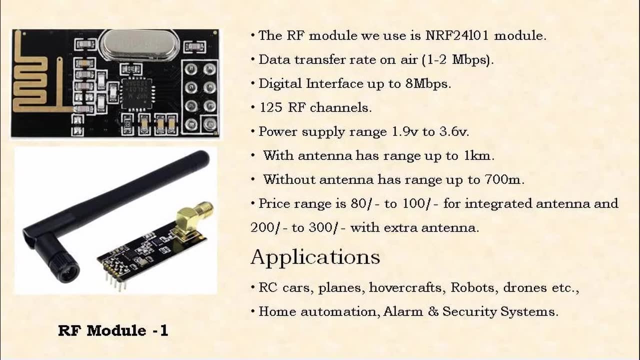 applications. this can be used in home security robots or automations. and that's all about wi-fi module. now we'll go to the next module. now we have come to the rf wireless transmission modules. this is one of my favorite and cheapest module available in rf, and the module i am showing you is the nrf24l01 module. 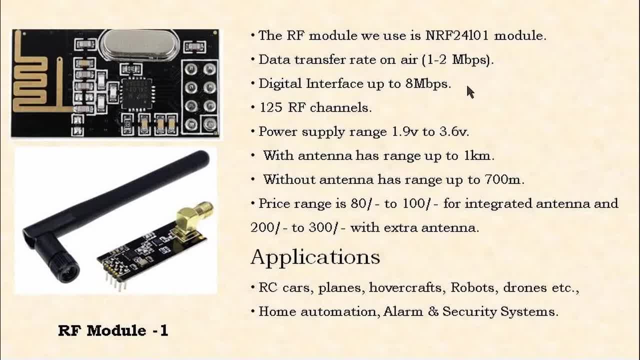 which is the cheapest and best and it has a data transfer rate on eight is one to two per second and digital interface up to eight mb per second. that means if we connect to the arduino and transmit the serial data, it can transfer more data than on air and using this module we can. 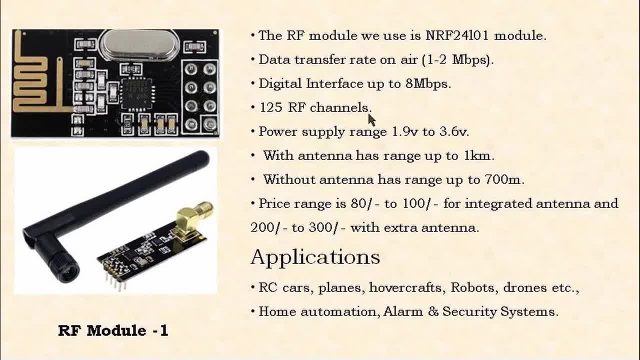 create 125 rf channels. that means we can make a multi-functional robot which has which, which has more features and it is a power. it has a power supply range of 1.9 volts to 3.6 volts. of course, we need a 3.3 voltage regulator to give the voltage to this, because 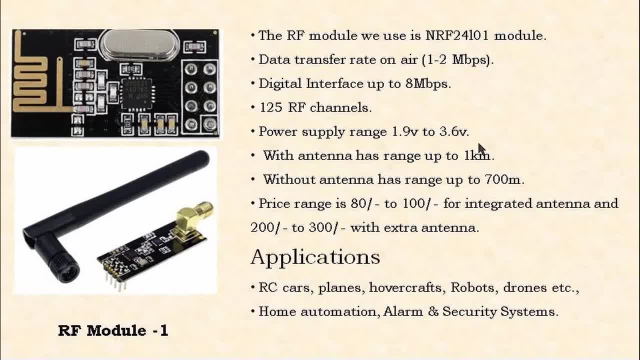 on arduino if we connect, if we operate using a battery. the 3.3 voltage from arduino is not sufficient because it doesn't give equal required amount of current to the nrf24l01 module. so we'll be using external power supply for this module with antenna. it has range of 3.6 volts to 3.6 volts. 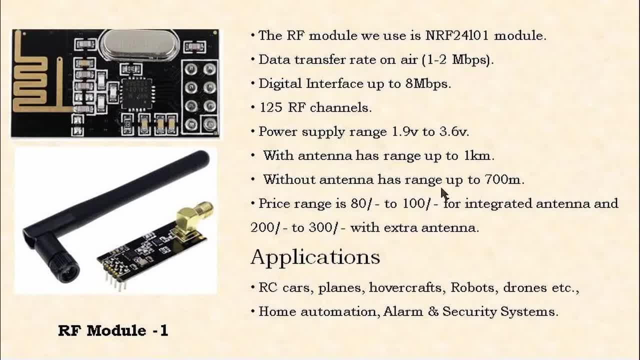 up to 1 kilometer without antenna. it has range up to 700 meters. that means the top module you see here has a integrated antenna. this module we have 700 meters range and with the pa plus lna that means extra antenna. it has a more range, up to one kilometer, and the price range is 80 to 100 rupees. 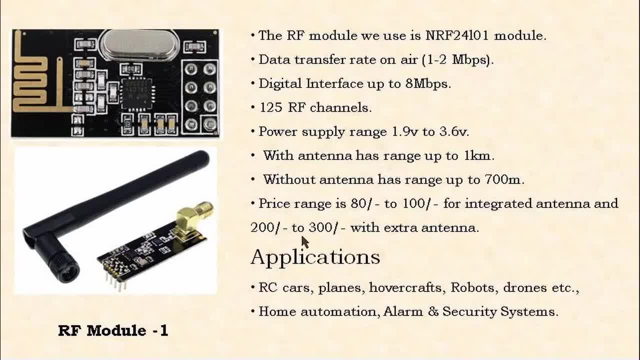 for integrated antenna and 200 rupees to 300 with extra antenna. that means this is the price range module is cheaper than this because it has a extra antenna, because that's why it is costly. and coming to the applications, as this is a radio frequency module, it has a number of applications. 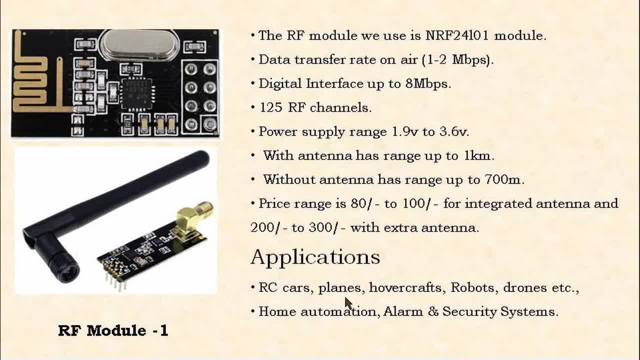 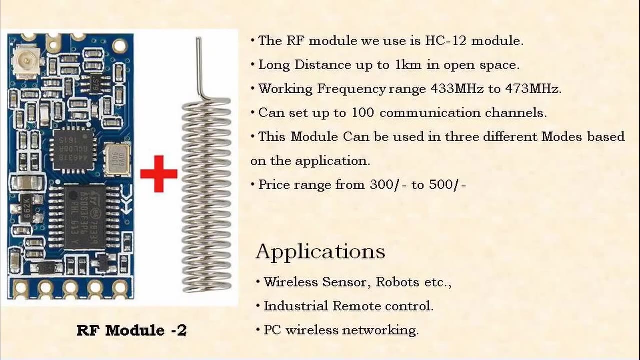 we can make toys, rc cars, planes, hovercrafts, robots, drones, etc will be make. i'll be making the projects on nrf24l0 module in future coming videos. and one more application is home machine alarm and security systems. the module i am showing you in this is a h312 module, which is a 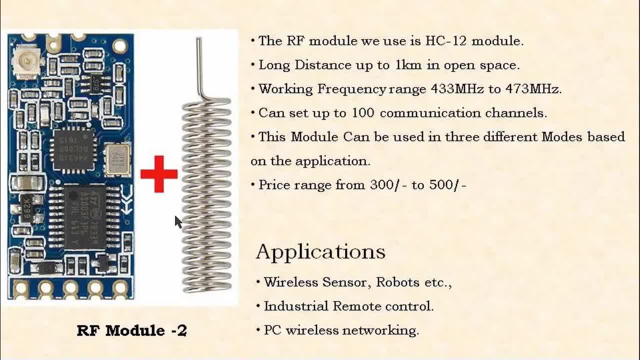 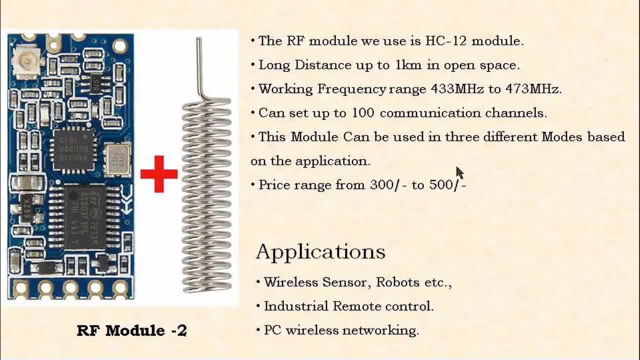 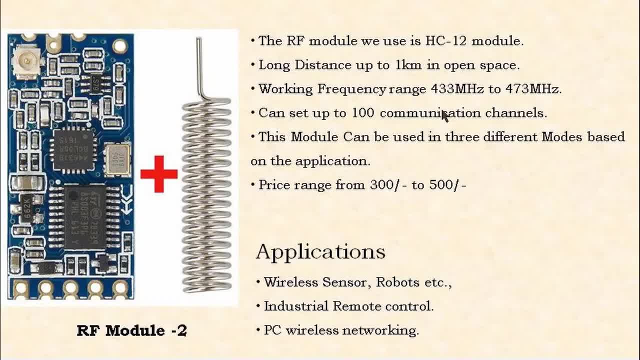 obstructed using the obstacles. whereas for 433 megahertz it can travel up to the long ranges with this frequency, and for this module it can can set up up to 100 communication channels. that means, uh, pretty much more, uh, lesser than nrf24l0. 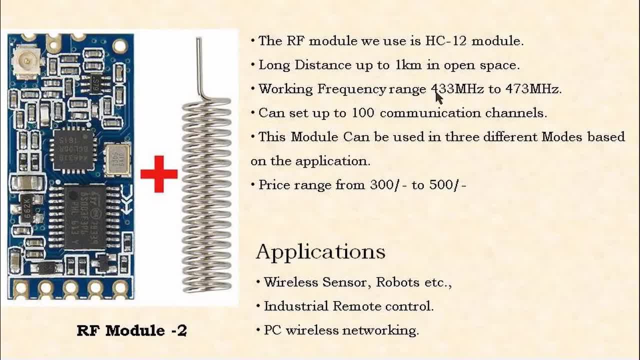 but it's good for uh. with a frequency of 433 megahertz, this module can be used in three different modes based on the application. that means if we vary the transmission power, the signal range is increased. that's how three different modes and price range is bit costlier than 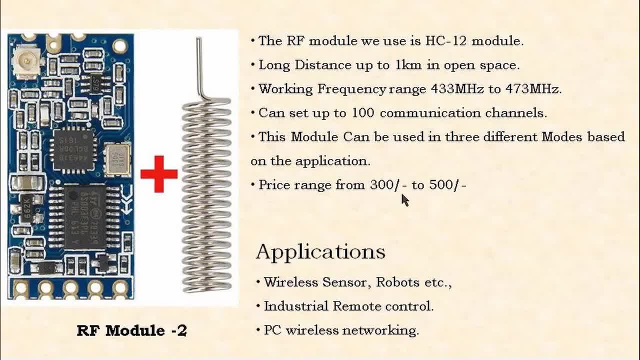 nrf24l01. that is 300 to 500 rupees. why i'm giving the price range is in different shops there is a different rate. in different shops there is a different rate. so i'll be giving you the average rate. and next is applications: is a wireless sensor, robots, etc. 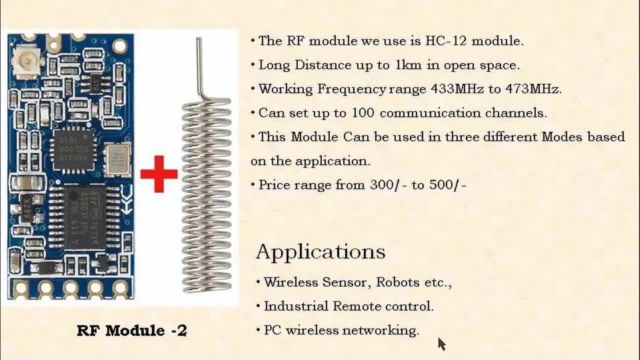 industrial remote control, pc wireless networking. and if you want to buy this, any any of these modules- the links are always given in the description below- you can straight away buy them. and that's all about hc12 module. now we'll go for next module. next is a zigbee xb module, which is a 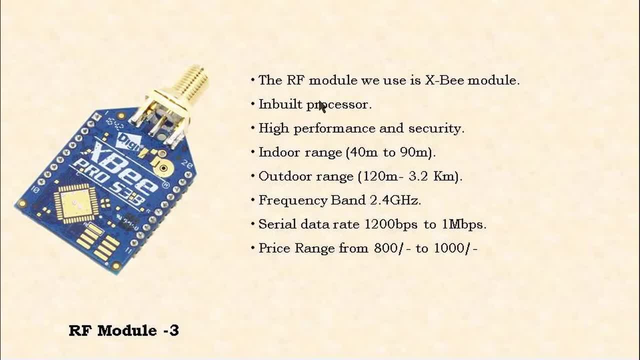 one type of rf module which is so powerful. also, the one thing is a good about this module is it has a inbuilt processor- the modules you have seen before: nrf24l01 or hc12 module. it requires arduino to process the you program, but xb doesn't require any processor, it can be programmed directly. 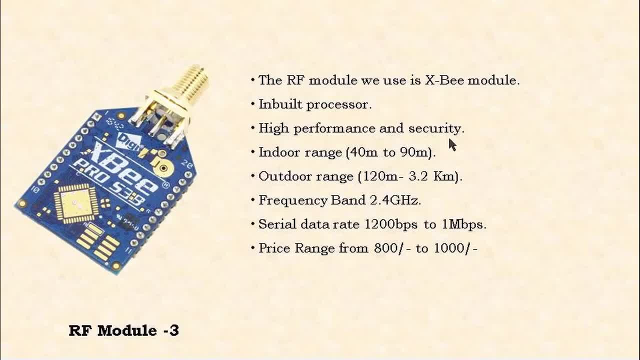 and it is a has a high performance and security also, and the range: coming to the range of this module, it has indoor range of 40 meters to 90 meters with the obstacle itself, and outdoor range of 120 meters to 3.2 kilometers. that's a bit long range and so it is a best module. 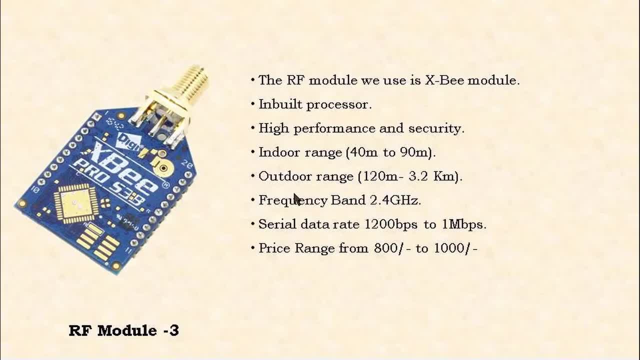 to transmit low data or sensor data or video data over long distances and frequency band and serial data rate: 1200 bytes per second to 1 mb per second. that means with the serial data rate you can say that you can send only some. that means low amount of data sometimes, simply basically. you can have maximum mass in the way of the data or equipment in the way of the data. this 새�is last. still, there is an issue aboutłącz slammed, and we also discussed how this one has the right or left leg to work. however, this one can only work. 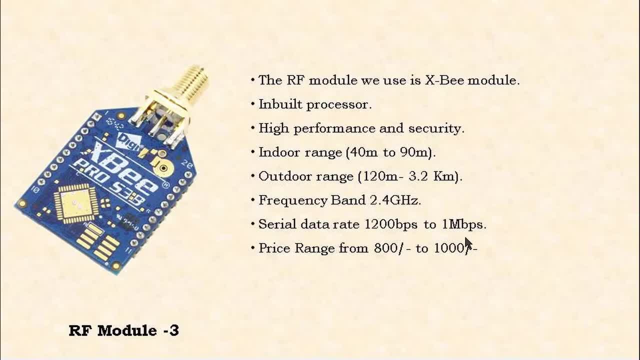 so most too. request too: change the audio on port. so most of the local emergencia on the port similar to this one, something if you want to send only some vertical running data without the Ultra-mode or components you just think is only a bit wrong. amount of data. sensor data can be transmitted using this XP module and 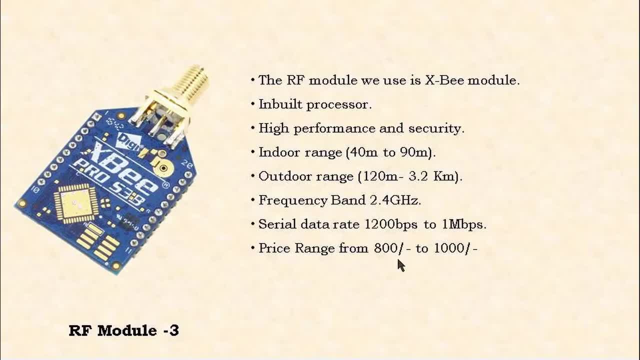 price ranges vary from 800 to 1000 rupees. because it has long range inbuilt processor, it is a bit costly, and that's all about XP. if we have a chance, if I have a chance, I'll make a demo on this XP, also the programming and all so now, 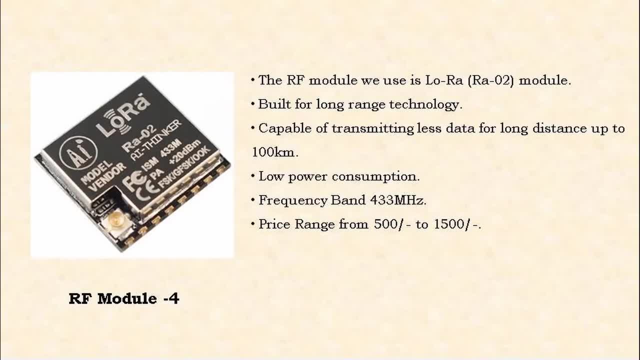 we will go to the next module. the next one is a LoRa module, which is a fourth type of module in our video. the name itself, LoRa, says that it is built for long range technology. it is capable of transmitting less data for long distance, up to 100 kilometers. that means because, suppose, say, temperature data or humidity.